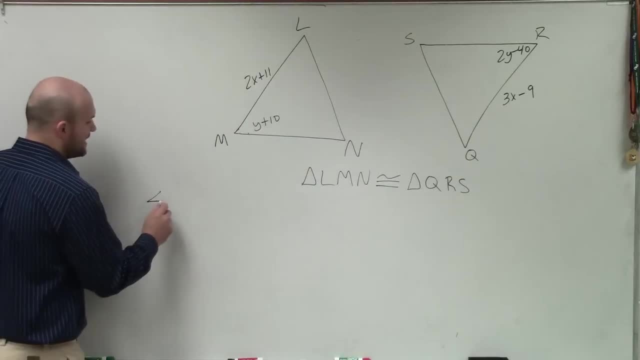 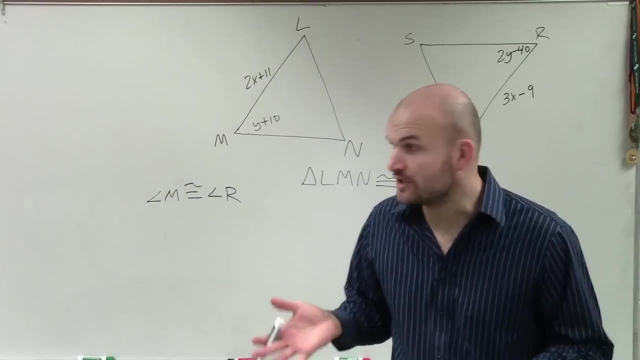 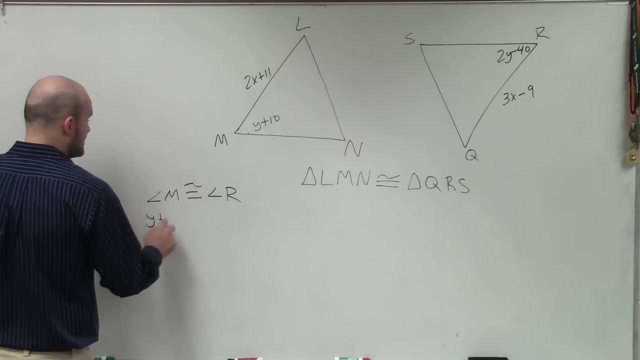 So therefore, by our congruency statement, we can determine that angle M is congruent to angle R. Since those angles are congruent, we know the measures of their angles have to be equal. So therefore I can just say: angle M is y plus 10 is equal to angle R. 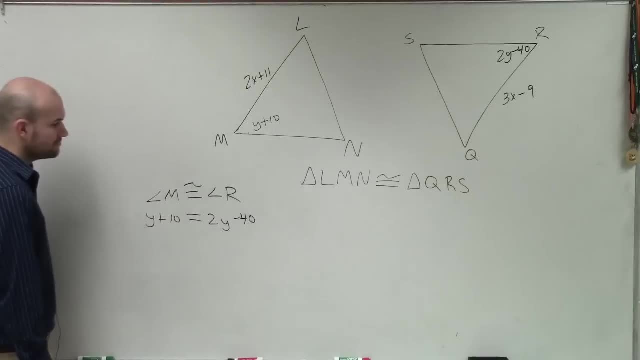 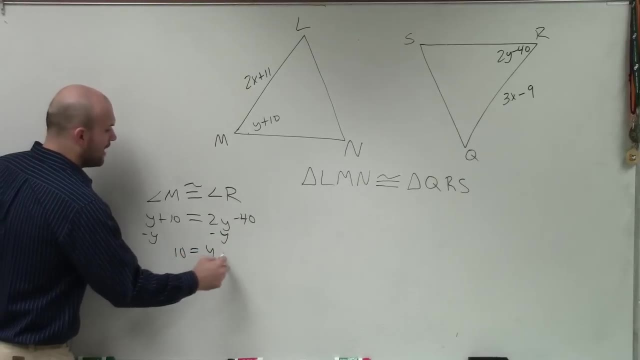 which is 2y minus 40.. Now I'm just going to simply solve for y, So I'll put the y's on the same side. So I have 10 equals y minus 40, add 40, add 40,. 50 equals y. But you have to just make sure. 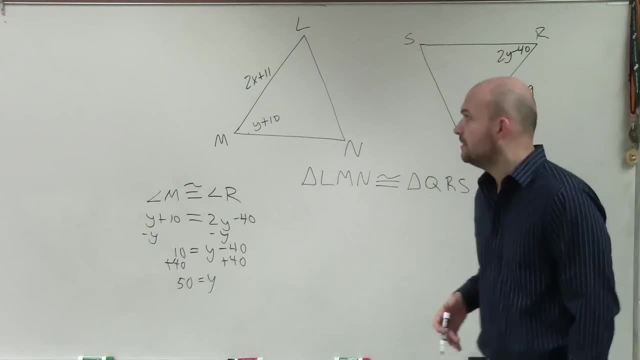 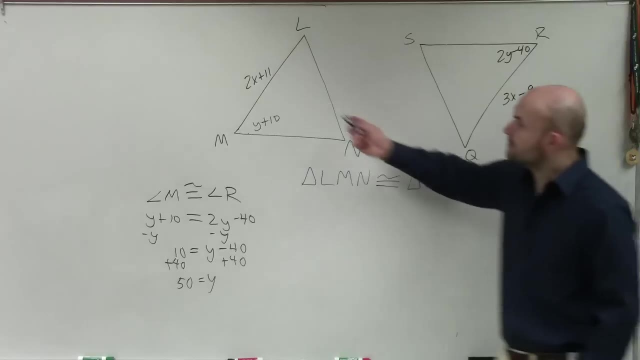 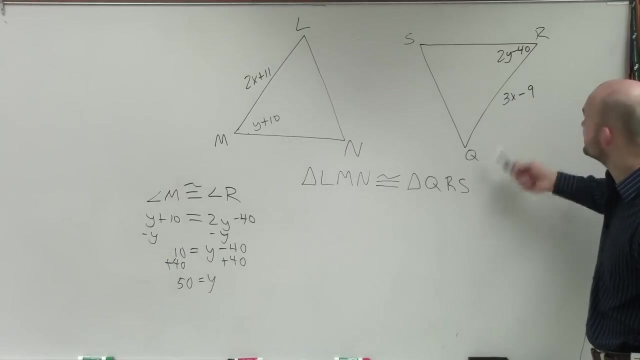 your angles are corresponding. before you can set that equation, They might not look like they're in the same spot or what they would be, so you have to look at your congruency statement. The next one is: we have ML Or LM. We want to be able to determine: is LM the same thing as QR? Well, notice this. 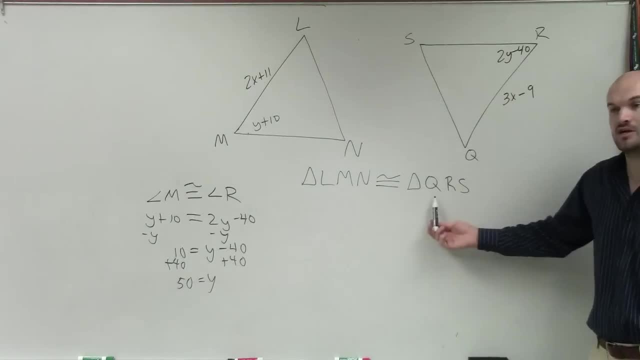 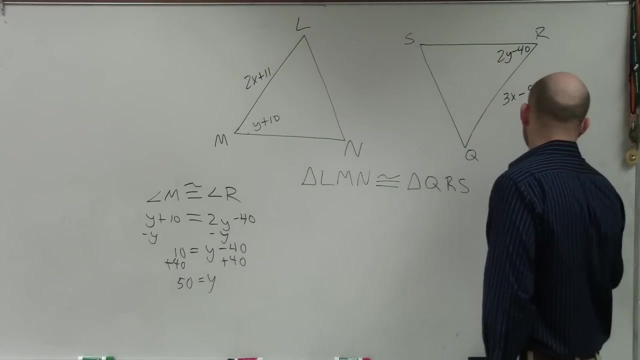 congruency statement starts with LM and this congruency starts with QR. We already know that M is congruent to R And therefore we can determine then that L is going to be congruent to Q. So, since I have LM is congruent to QR, we can now write a congruency statement that 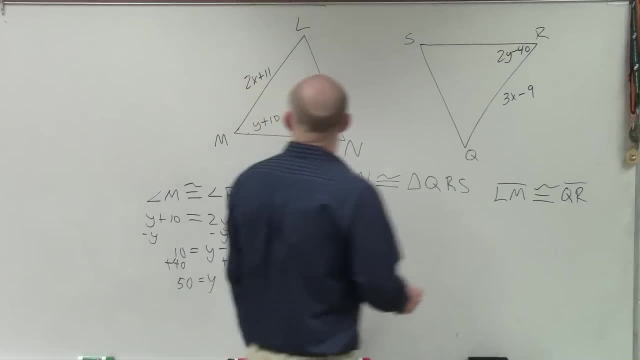 the lengths of those sets are congruent to Q. So we can now write a congruency statement that when the lengths of those sets are congruent to QR, we can now write a congruency statement that when the links of those sets are congruent to Q. So if we look at the next slide, we 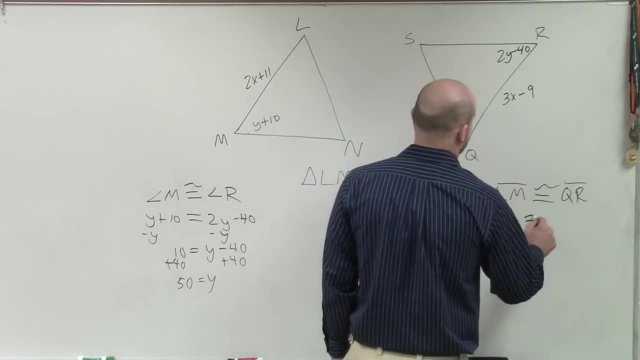 can see that the lengths of those sets are congruent to Q, Then the lengths of those sets are congruent to QR. So, coincidentally, L and QR are congruent to both sides, but these two sides are also equal in measure. So therefore I can say now that 2x plus 11. 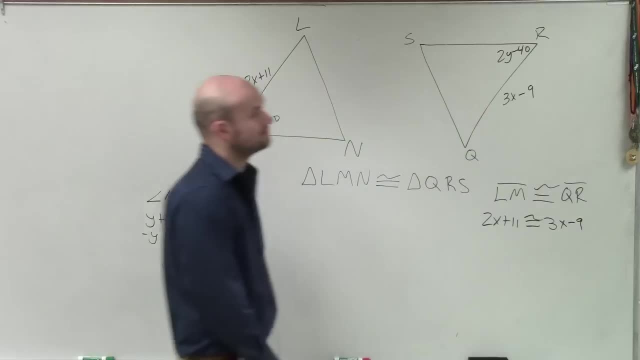 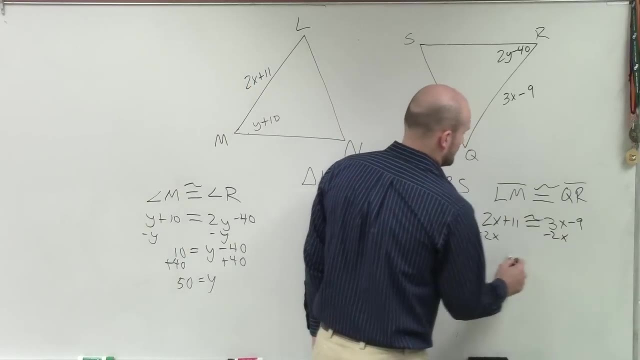 is congruent to 3x minus 9.. Now we just need to solve for x again, So we get the x's to the same side And I have 11 is equal. I'll just write that as an equal: 11 equals x. 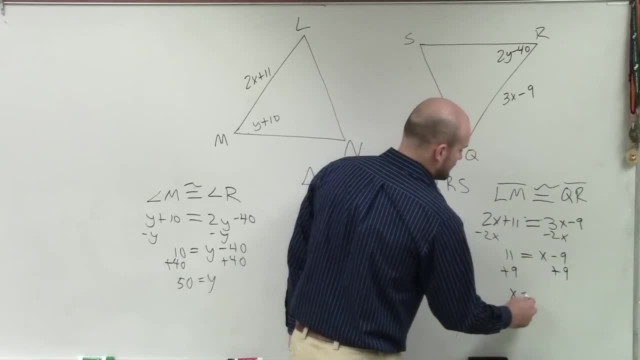 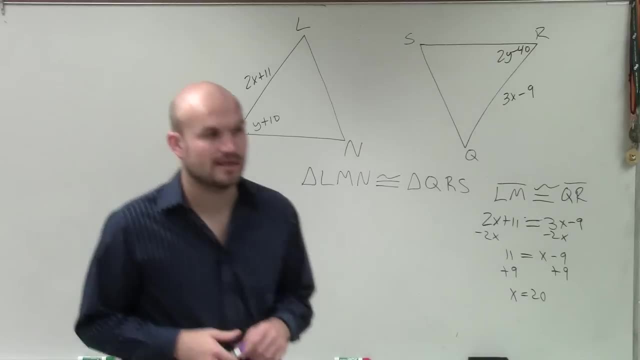 minus 9,, add the 9,, x equals 20.. So, therefore, your values for y should be more than or equal to q. Now you can fill in your values for y, So you'll notice that you're going to have should be 50, and x is for 20.. Cool, Make sense Kind of, Maybe a little bit.